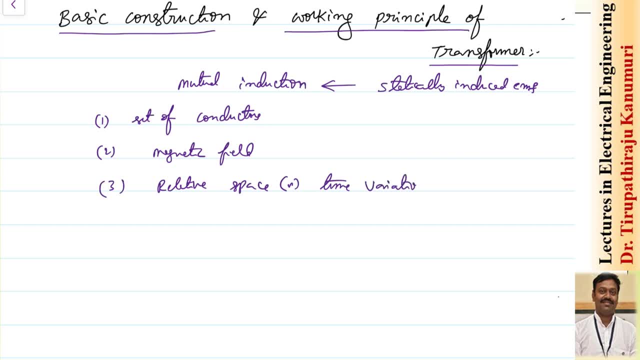 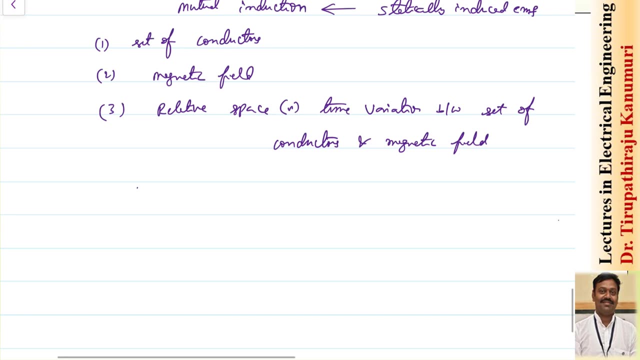 time variation between the set of conductors and the magnetic field. So, as per the Faraday's laws of electromagnetic induction, the Faraday has stated that the emf induced is directly proportional to rate of change of flux linkages. It stated that it will be directly proportional to rate of change of flux linkages. So, flux linkages. 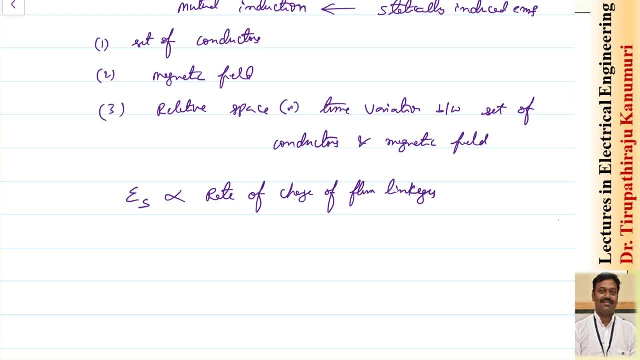 should change. So this is possible by using two methods: Either the magnetic field is stationary and the conductors are moving, or, second, that is called as a dynamically induced emf, because conductors are moving. and the second option is the conductors are stationary and the magnetic field 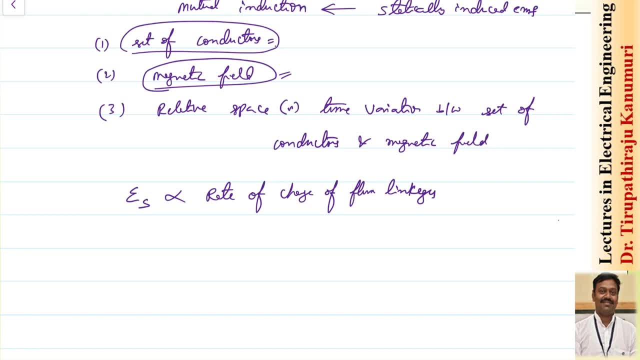 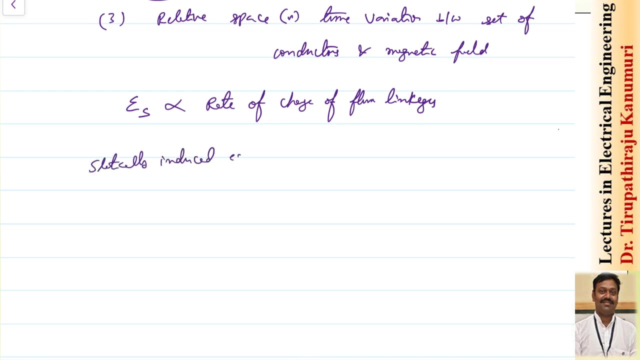 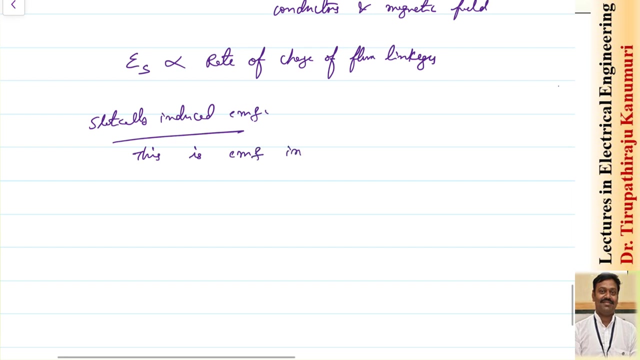 varies with respect to time, As the conductors are stationary. that's why it is called as statically induced emf. That's why it is called as the statically induced emf. So what is statically induced emf? So statically induced emf. So this is emf induced in a set of stationary conductors. 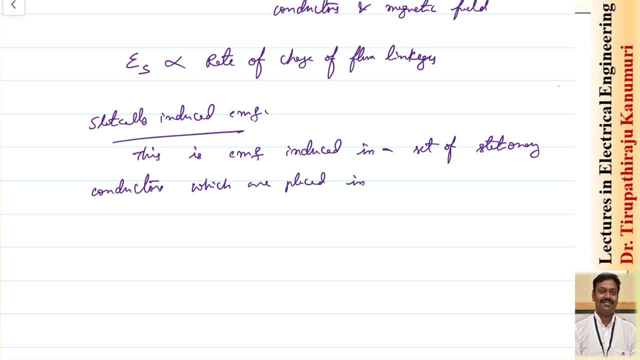 which are placed in time, varying magnetic field. So let us take, for example, I am taking some conductor having N turns. Let us assume they are linking some flux phi, So flux phi is passing through them. This flux is changing with respect to time, So the emf equation it is stating that it is. 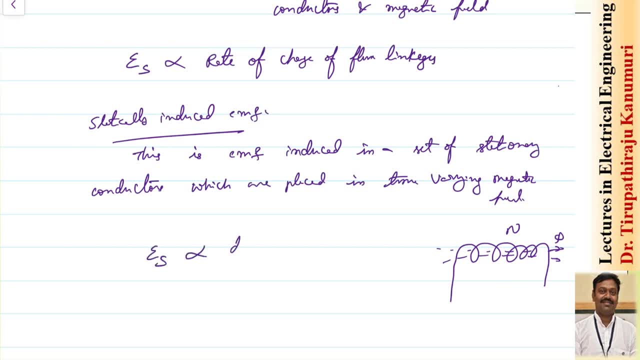 proportional to rate of change of flux linkages, because rate of flux is changing with respect to time change. the flux is changing with respect to time. so this is d by dt of the flux linkages. the flux you can see phi is linking with each turn of the coil. total link is linking with n turns. so total. 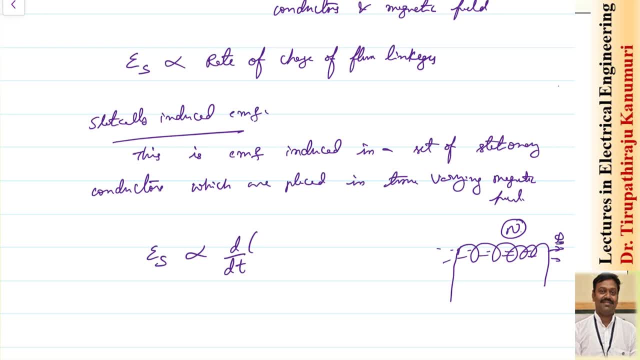 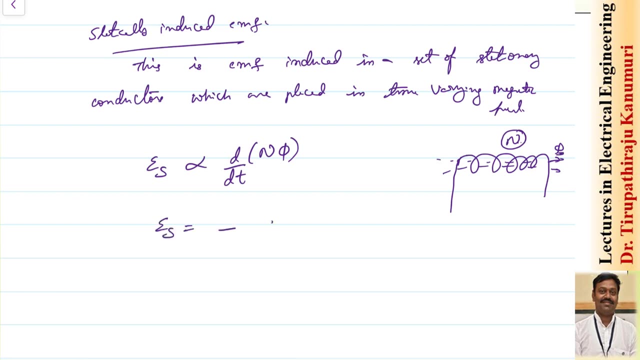 flux linkages is: each turn is linking a flux of phi and total there are n turns. so that's why this will be number of turns multiplied by flux linking each turn. so this is equal to d by dt of n phi, and this self-induced emf is given by the negative sign of the d by dt of n phi. so this d by dt of n. 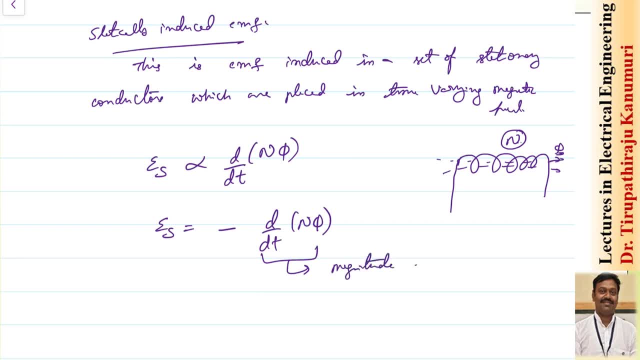 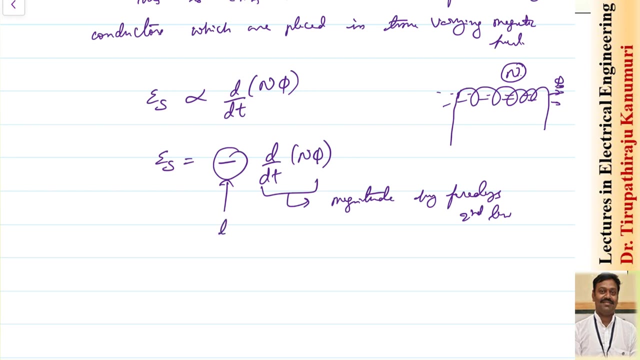 phi. this gives the magnitude of the emf. so this is given by the faraday's second law and this negative sign indicates so whatever the emf will induced that will oppose the cause or that will oppose your supply voltage. so this is given by the lenz's law. 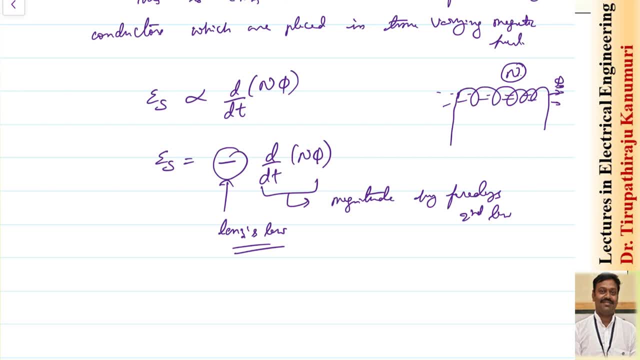 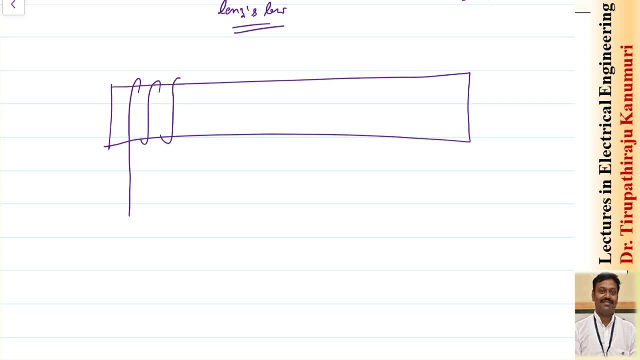 so i am taking an iron core on this. i am making one coil. this is the first coil. let us assume the coil is coil a, having n1 turns. let us assume there is one more coil which is kept here on the same iron core. so this is having n two turns. let us take it as coil number b. so now let us assume 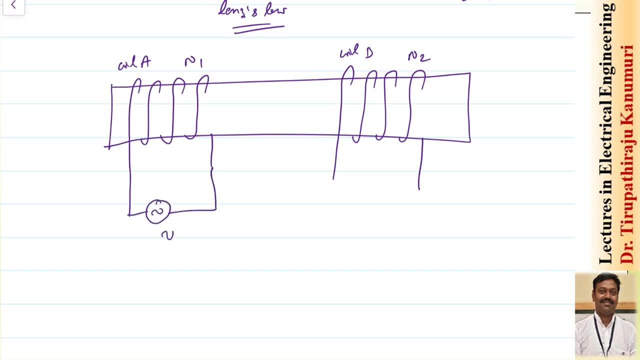 let us assume this coil one is connected to sinusoidal supply or sinusoidal voltage given by vi. so whenever vi is given to a coil because we have, it is like nothing but an inductor. whenever inductor connected to sinusoidal supply, we know the current will pass through it. that current 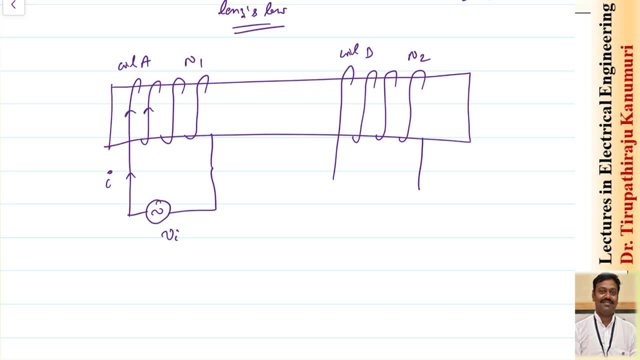 let us take it as i. so whenever the current is passing like this, because the current is passing like this so it will produce a flux. so the direction of the flux can be found by using the right hand thumb rule, where you hold your coil with your right hand. in such a way, your 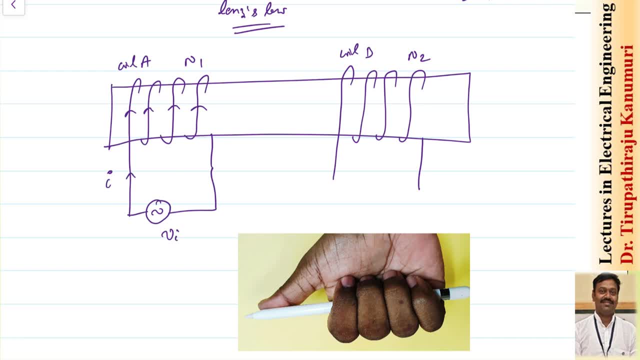 curl finger indicates the direction of the current, then your thumb indicates the direction of the magnetic field. so if you apply your right hand thumb rule, you will observe that your flux lines will come like this: this will be the direction of the flux lines and the flux lines. 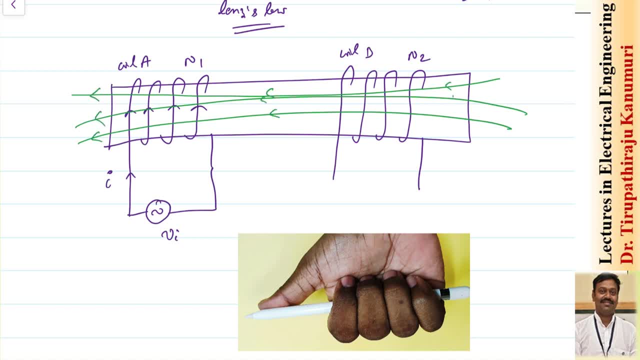 will come out like this: this is my direction of the flux lines. so this is my direction of the flux. so as the current is changing with respect to time, the flux also changes with respect to time. so now you can see, this flux is linking with both this coil number a, as well as coil b. it is linking both the coils. so as it is linking both the coils, 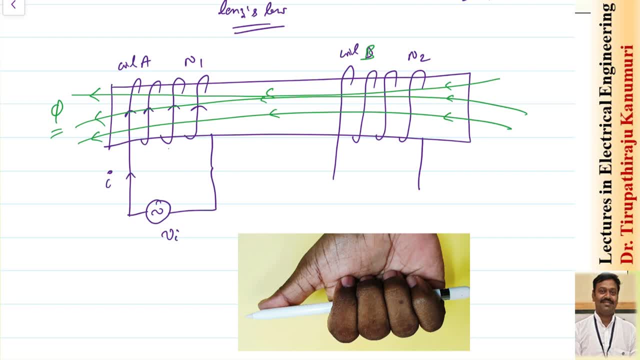 because, as for the faraday's law, it will induce the emf in both the coils. the emf induced in the first coil is due to the flux of the same coil, so that's why it is called as a self-induced emf, and the emf induced in the second coil due to the flux produced by the first coil. 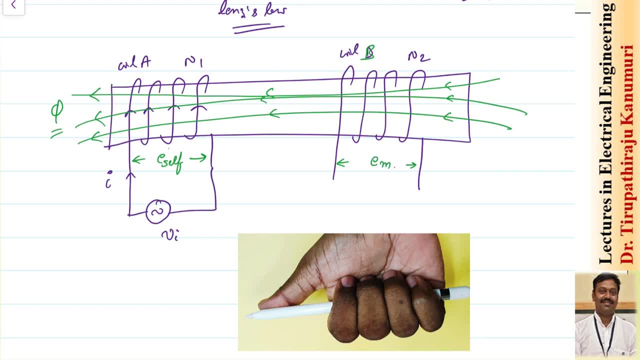 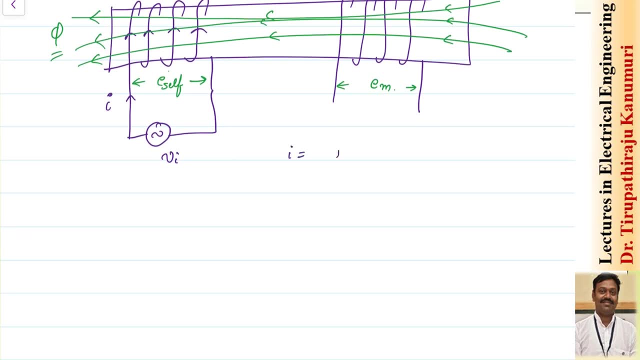 this is called as the mutually induced emf. this is called as the mutually induced emf or represented by the term e suffix m, e suffix m. okay, let us proceed further. so let us assume the current equation. i am taking as i maximum sine omega t, so the force that is responsible for the production of the flux. 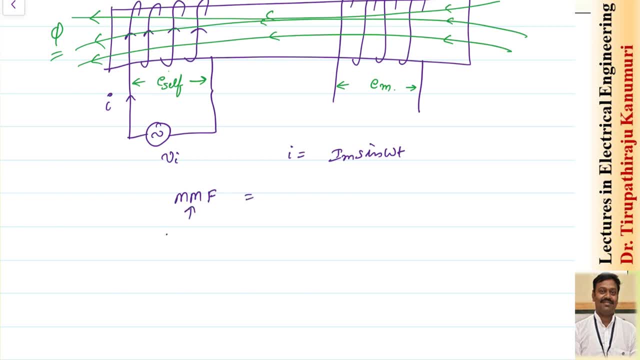 is called as the magneto motive force. this is called as magneto motive force. it is just similar to electromotive force, which is responsible for movement of the current. so it is a constant in electrical engineering which is responsible for production of the current. same thing for the production of the magnetic flux, the force that 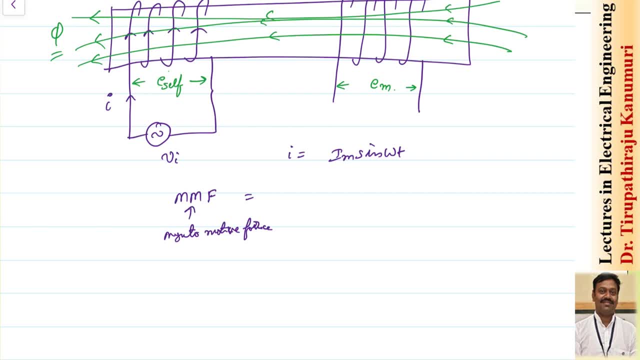 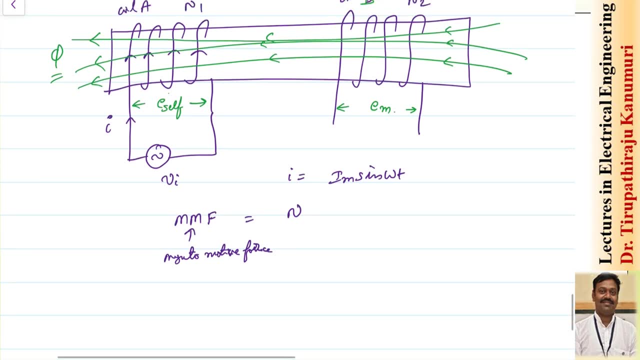 is required is called as magneto motive force. this is called as magneto motive force. this will be equal to the number of turns through which the current is passing, the number of turns the current is passing through the first coil. so number of turns is equal to n1 and the current passing 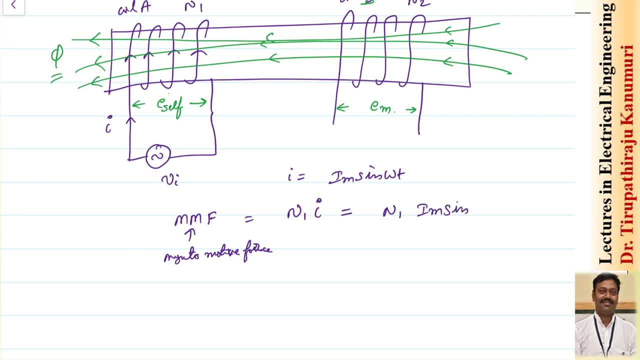 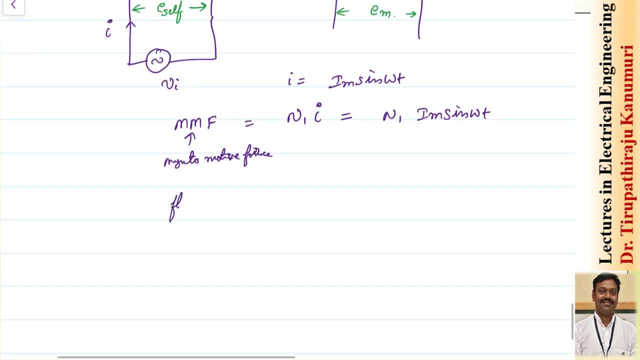 through this coil, is i? so this i can write as n1 into, so you can see that the mmf is also varying with respect to time. so now if you want to calculate the flux, so the flux will be equal to magneto motive force divided by reluctance of your. 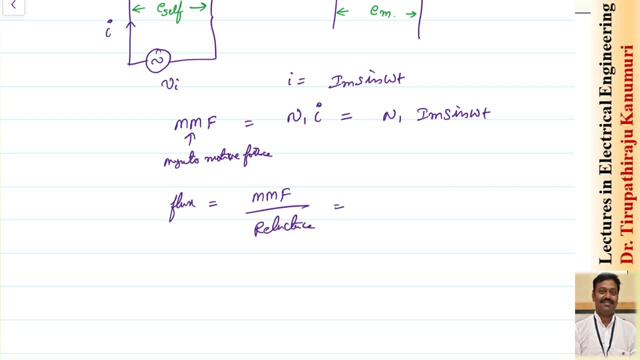 magnetic circuit because ideally the reluctance should be equal to zero. that means without giving any current the flux should come. but practically there will be some finite permeability of the core. that means the core, the permeability or relative permeability of the core will not be equal to. 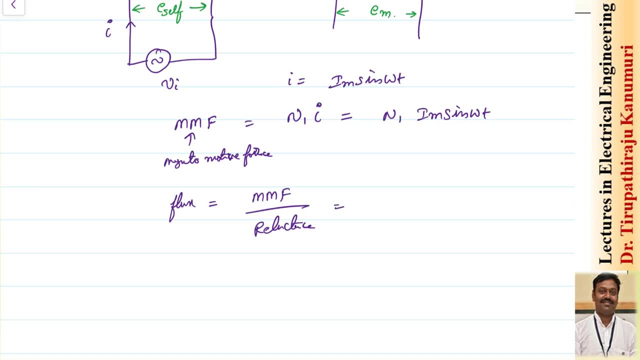 infinite. always some current is required to produce the flux, so that's why the reluctance is always finite. so we can tell this as n1 i maximum sine omega t divided by. let us represent the reluctance by letter r, so this term n1 i maximum by r. so this i can take as phi maximum. 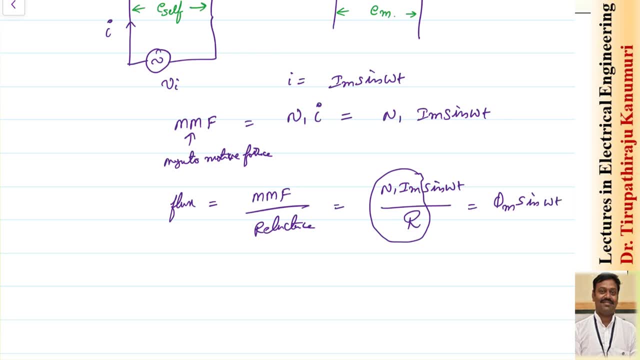 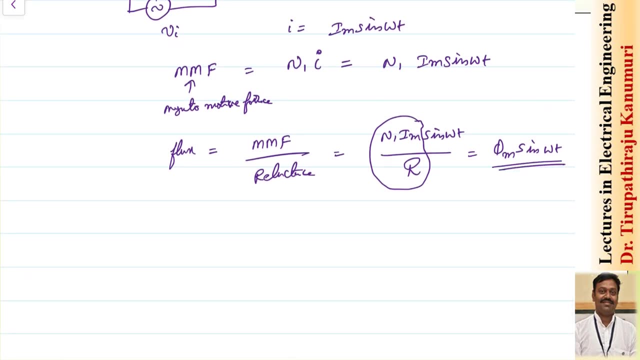 remaining term i am taking out this will be equal to phi maximum sine omega t. so because of this phi sine omega t, the flux is linking both the primary turns. that means the turns of the coil number one and the turns of the coil number two. because of this, the emf induced in the first coil. so that is called as. 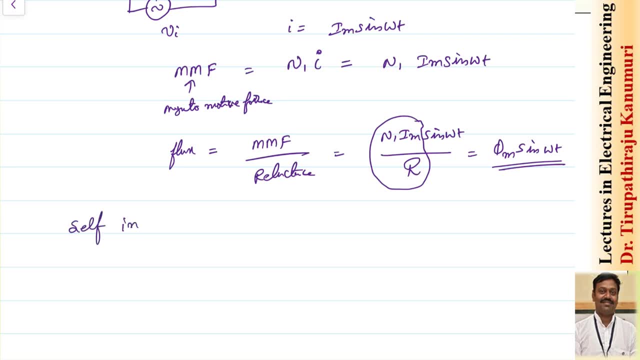 self-induced emf. so i am defining the term self-induced emf. is this self-induced emf? is the emf induced in a coil due to time varying nature of current flowing through its own coil? because of time varying nature of current flowing through its own coil, the emf is 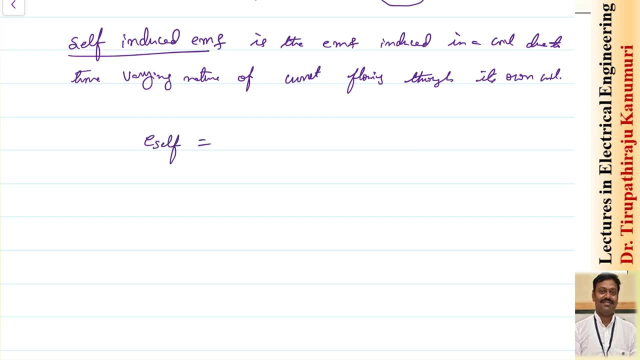 induced that emf- i am defining by the term e self- will be equal to minus d by dt of how many number of turns are there? n1 turns are there. each turn is linking with the flux of t, so this is the flux of V because the number of turns are constant. so I can take it as minus m 1 into this d phi by dt and 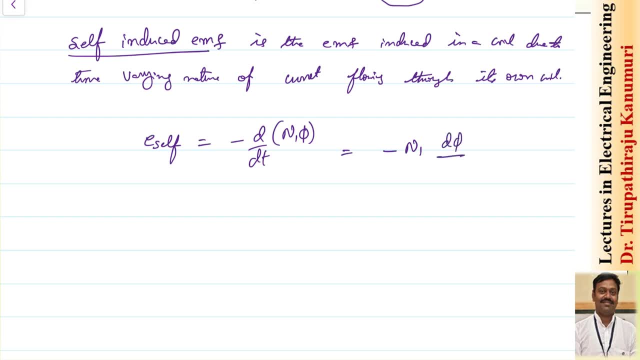 dusty dividing and multiplying with di1. so this will be defy by di 1 multiplied by di 1 by oO, because we know the current i-one is changing with respect to time, the current that is given to the first coil i am representing by i suffix 1, so this term I can separate out. so this term is called as the. 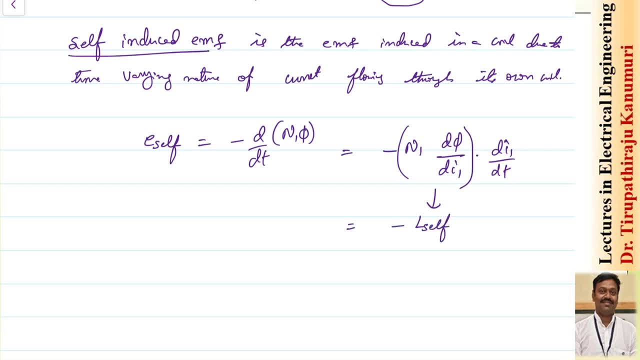 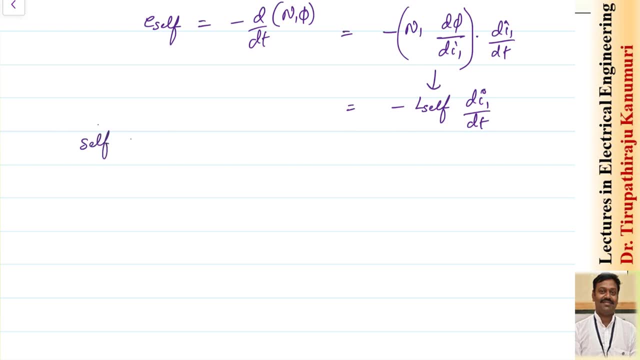 self inductance of your coil. So this can be represented by minus L self into di1 by dt. So this L self is called as the self inductance. This is called as the self inductance, which is also called as L self of a coil, is the rate of change of, because n can be taken. 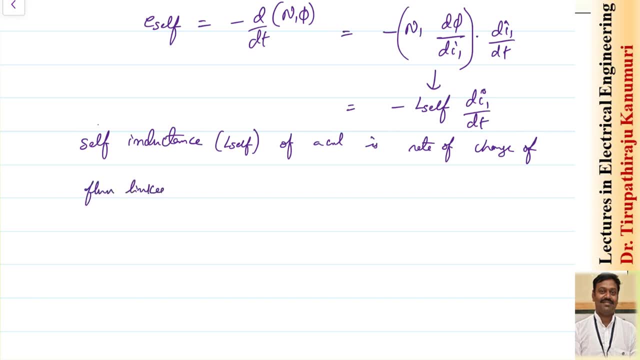 inside rate of change of flux linkages of a coil due to time varying nature of current flowing through its own coil. because it is equal to d by di1 of n1 multiplied by 1 by dt, So it is equal to the rate of change of flux linkages of a coil due to time varying. 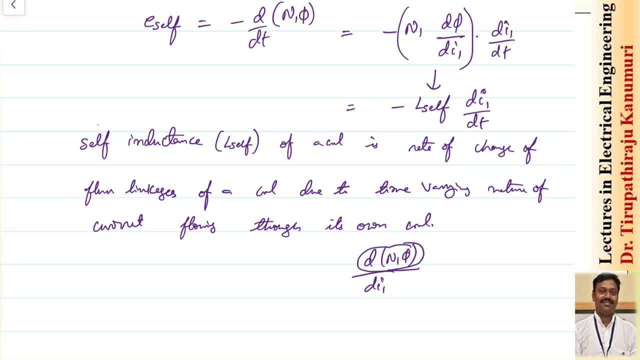 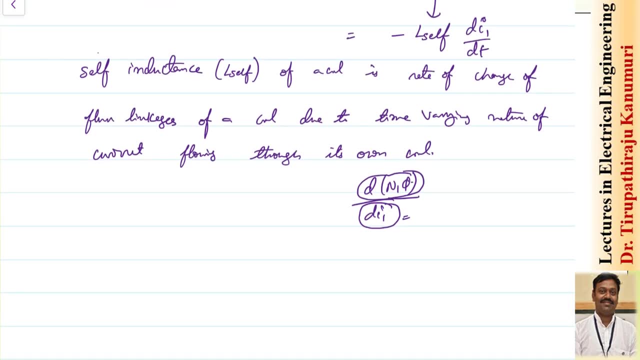 multiplied by 5.. So this is the rate of change of the flux linkages due to the change in the current in the primary or the current that is passing through the same coil is changing, So this is called as the self-inductance of a coil. So now the self-induced DMF, because we 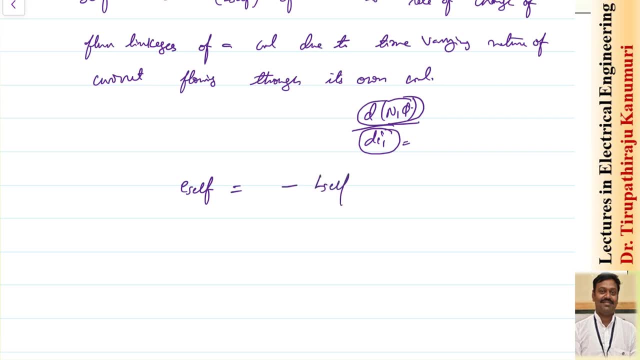 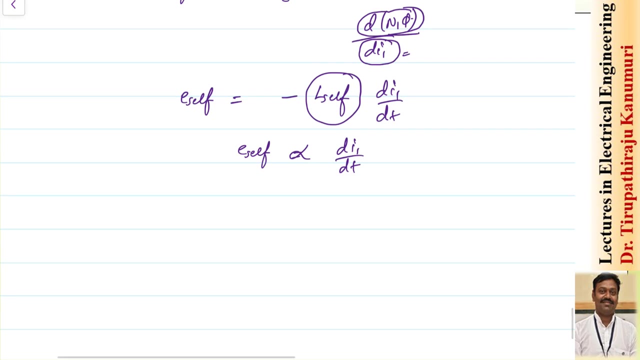 have seen here it is given by minus L self into di1 by dt. So L self is the property of the coil, it is constant. So we can tell the self-induced DMF is proportional to di1 by dt. It is proportional to di1 by dt and the negative sign indicates it always opposes your cause, always opposes the. 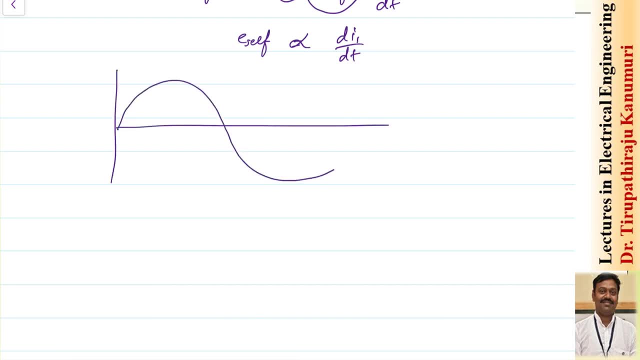 cause. So practically, if you take- let us assume this is my supply voltage, So this is I am taking by vi. We are going to prove in the coming class, whatever the EMF is produced that will oppose the cause. So that is why the EMF that is induced will be. 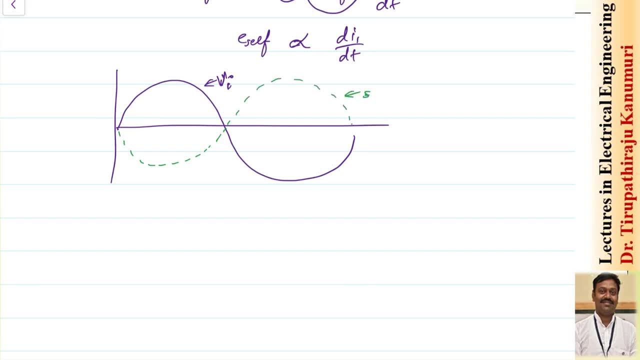 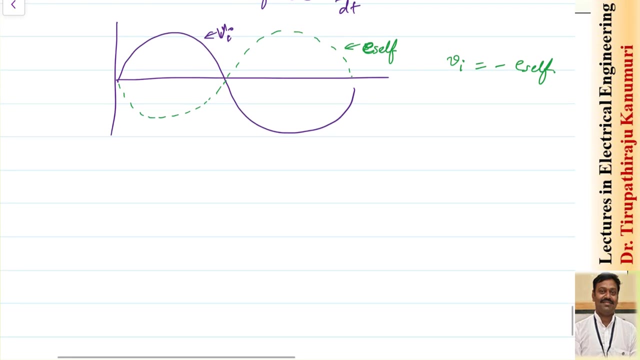 180 degrees opposite to the applied voltage. This is my E self-induced EMF. So self-induced EMF will be 180 degrees opposite to your supply voltage. That means we can tell that the input voltage will be equal to minus E self. It is opposite to self-induced EMF. So now there is 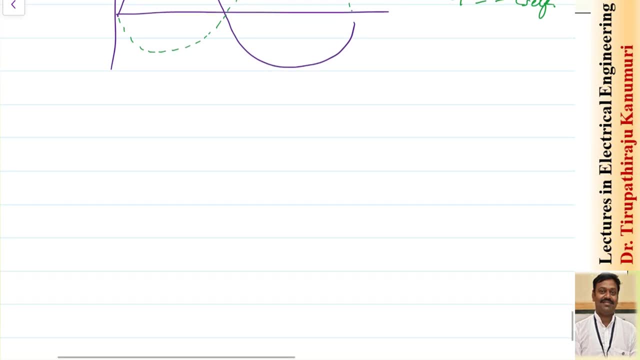 one more term, because this flux is linking with the second coil. also because of that, the EMF will be induced in the second coil, which is given by EM will be equal to minus L self into di1 by dt. So this is my self-induced EMF. So now there is one more term. 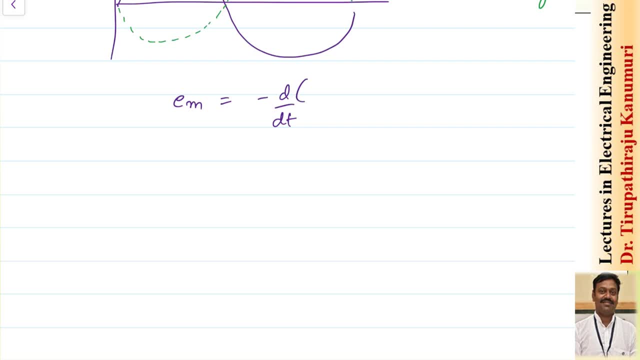 minus d by dt, of that flux is linking with n2- number of turns and each turn is linking a flux of phi. This phi is produced by the first coil. So this I can rearrange, minus n2 is constant. So I am taking out, So I am multiplying and dividing with di1.. This will be d5 by di1 multiplied by. 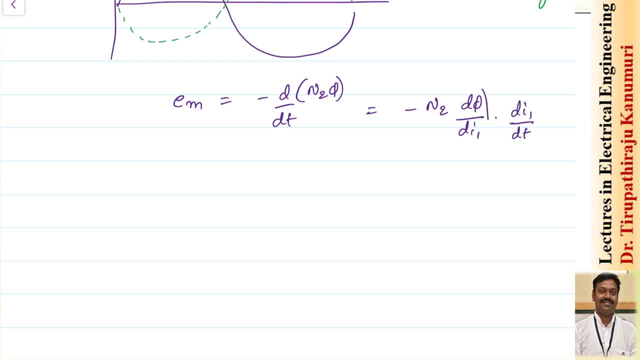 di1 by dt Getting it. So again this term. you can see here this is the flux linkages of the second coil because coil turns are in the second coil. So this is the flux linkages of the second. coil turns are having n2 due to time varying nature of current passing through the first coil. 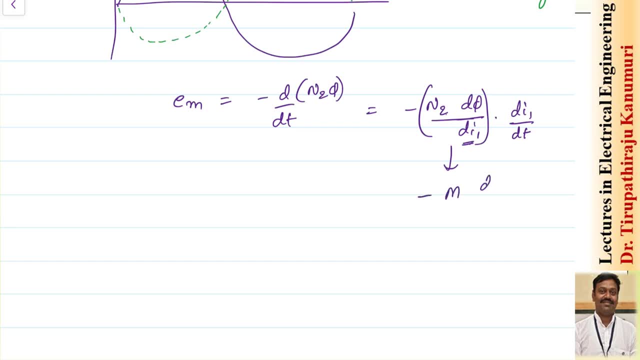 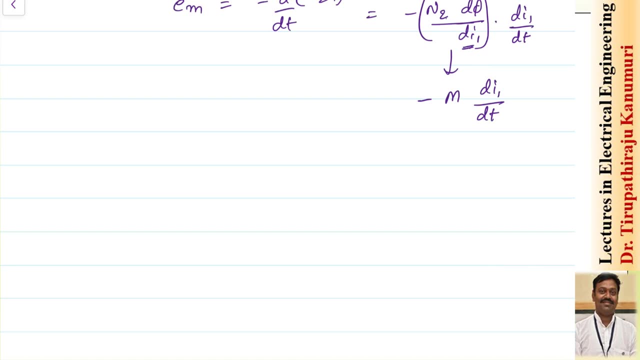 which is defined by the term called as mutual inductance. It is a property of the coil multiplied by di1, by dt Again. if you want the further details of what is this mutual induction, inductance and all these terms I have discussed in the EMF lectures, you can please refer to my 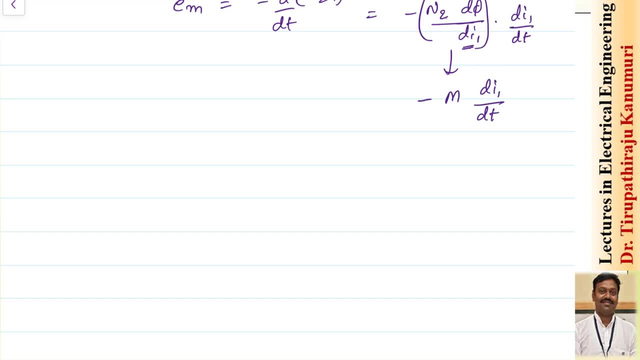 EMFT lectures. So there, I have discussed this in detail in the magnetic circuits. So now let us proceed further. what is this m? So this m is called as the mutual inductance. So this mutual inductance between two coils may be defined as rate of change of flux linkages at a coil with respect to the 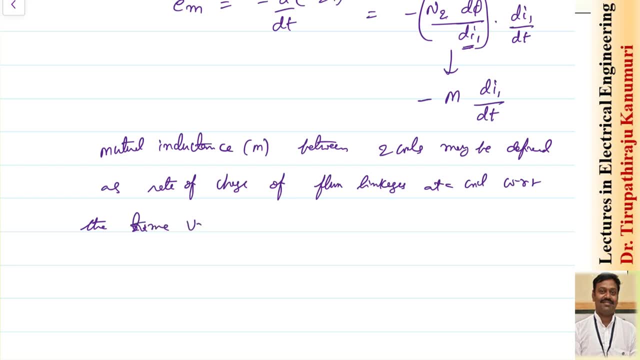 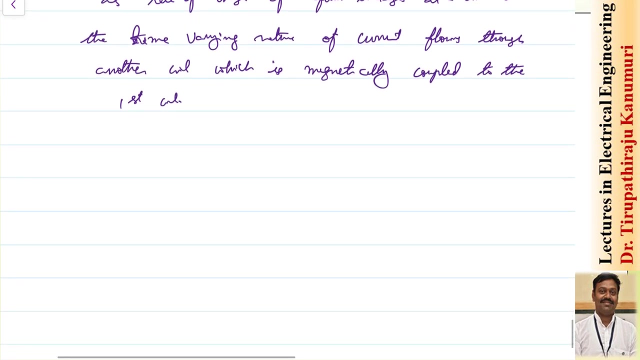 Time varying nature of current flowing through another coil which is magnetically coupled to the first coil. So current is passing through some other coil which is coupled to this first coil. Again you can see this mutually induced EMF is also coming as a minus sign. 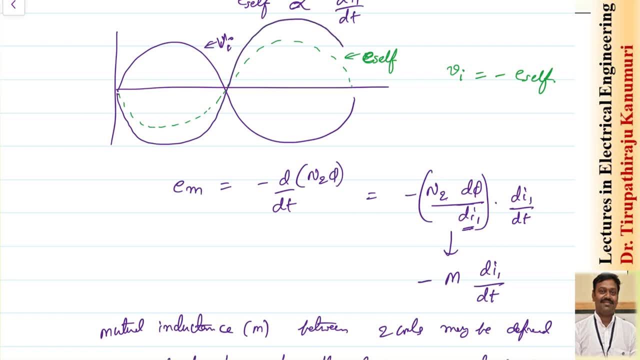 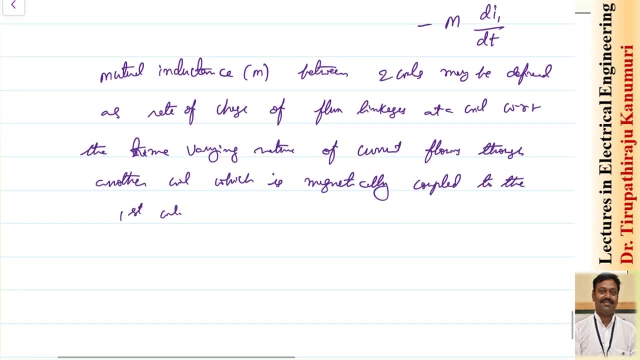 So this mutually induced EMF will also oppose the cause, or this mutually induced EMF will be in phase with the self induced EMF. So this is given by EM. So now there is one more thing that we have to learn before going to the transformers. 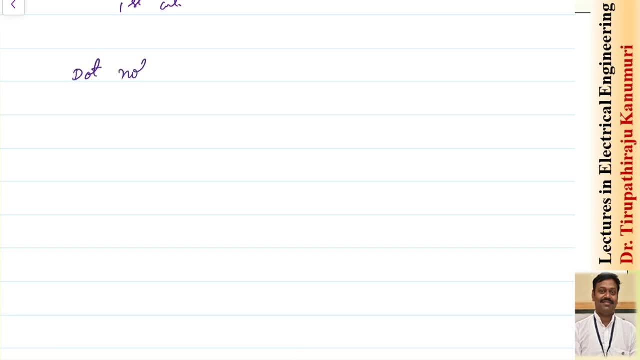 that is the dot notation. So the dot notation is: Let us assume I am taking a transformer core, So on which the two coils are one. So let us assume this is my second coil. So here the dot is represented on the coil. 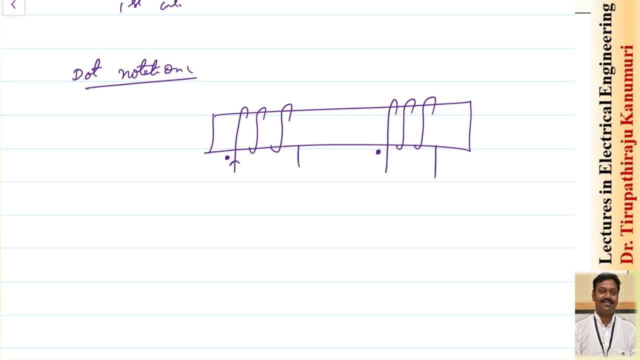 So if the current enters the dot of both the coils- That means the current entering or leaving the dot of both the coils- Then we can tell the flux produced by them will add to each other. So that is called, as the fluxes are adding to each other or they are positively coupled. 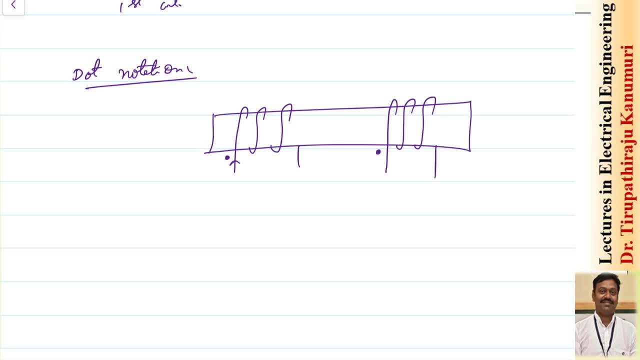 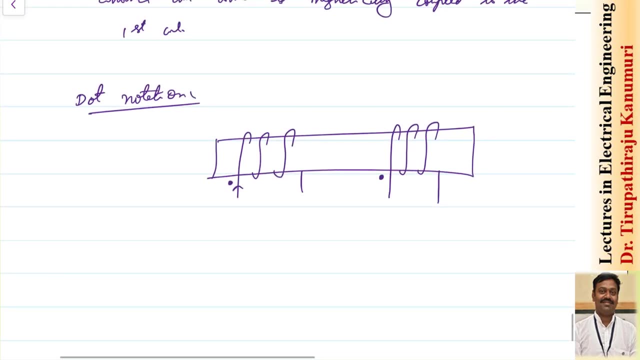 The major reason Using the dot notation is to predict what will be the orientation of the flux internally, How the flux will pass internally. Let us take this case. So first I am taking this coil number A, or coil A, having N turns and coil B is having 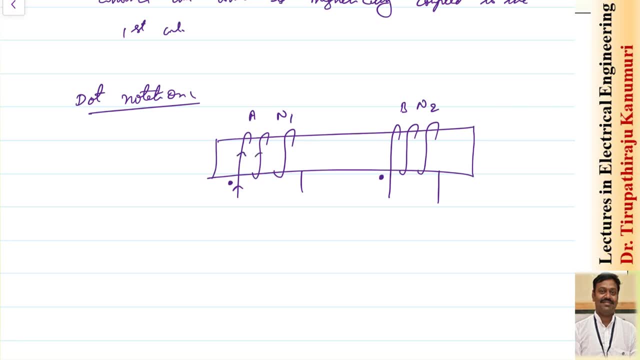 N2 turns. Let us assume the flux is passing. current is passing like this. when the current is passing like this, If you apply your right hand thumb rule, the direction of the flux produced by this will be like this: This is the direction of the flux produced by this. 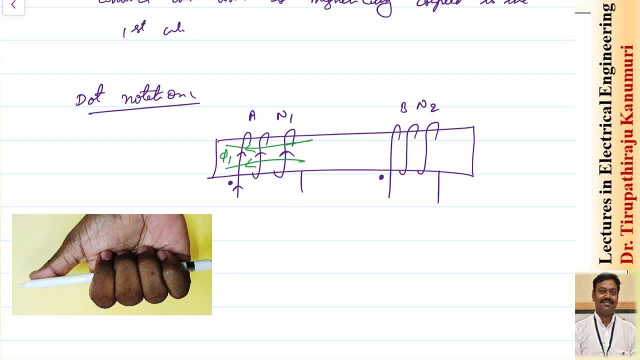 Let us take it as flux phi1.. Similarly, In order To aid the same direction of the flux, the current should pass in the second coil in such a way that the flux produced will be in the same direction, The flux produced by this also in the same direction or in a common magnetic circuit. 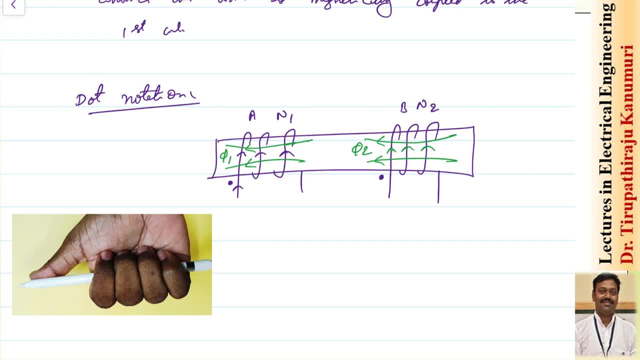 both phi A and phi B or phi 1 and phi 2 will add to each other, Then they are called as positively coupled. So in order to make the positively coupled, if the current is entering the dot here, the current should enter the dot of the second coil. 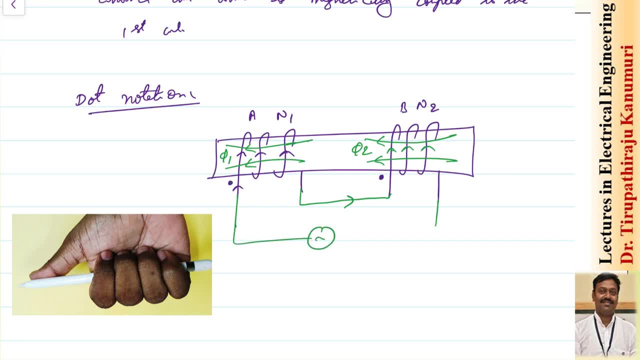 How can we make it? We can connect like this. So this I am connecting to external supply, Because the current is entering the dot of both the coils or leaving both the coils. then we tell that the magnetic flux inside is magnetically aiding to each other. 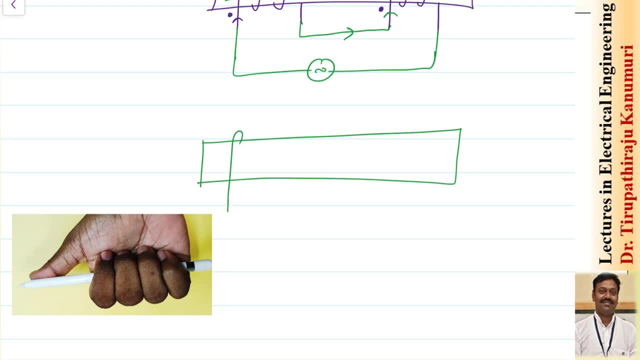 Let us assume the current enters So same coil. I am just making the winding, So the dot notation is here. dot notation is here. So let us assume the current is entering the dot of one coil and leaving the dot of another coil. The current is entering from the other side. 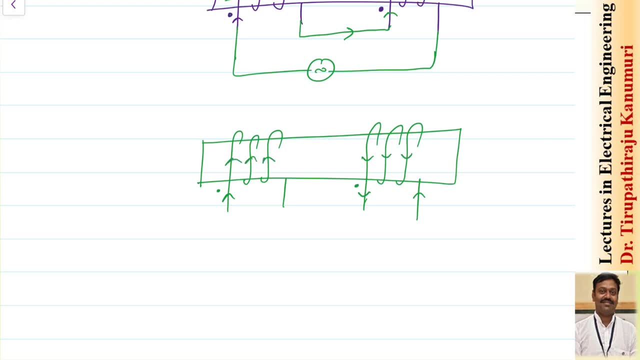 So the current direction will be like this here. Current direction will be like this here: If you draw the flux path for this one, the flux produced by this one will be like this: This is my flux, phi A- and the flux produced by the second one will be in the opposite. 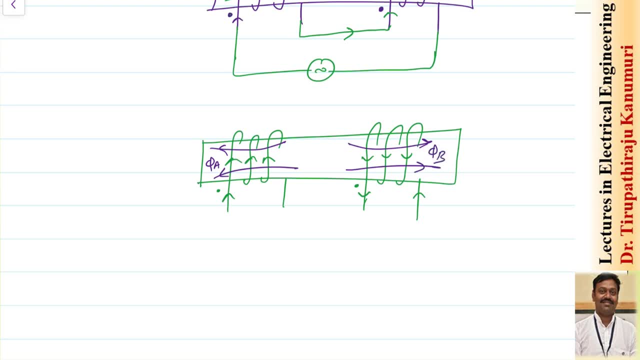 direction You can see. this is my flux, produced by the second coil. That means if the current is entering the dot of one coil and leaving the dot of another coil, then in a common magnetic circuit the flux will be opposed to each other, Or we call that they are negatively coupled. 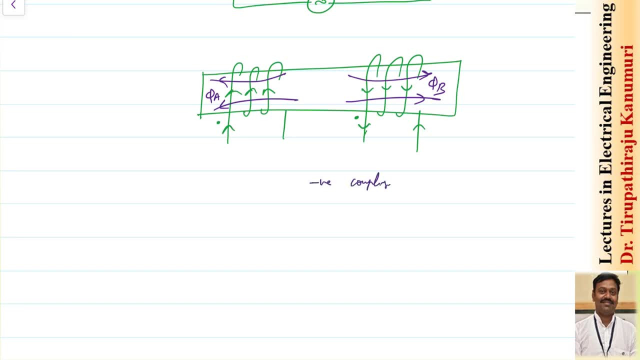 That coupling is called as negative coupling. Negative coupling means the flux is opposing each other. Let us make one connection: how to get it? So if this is my supply, the current is entering like this: So whatever is coming out, make the connection like this: 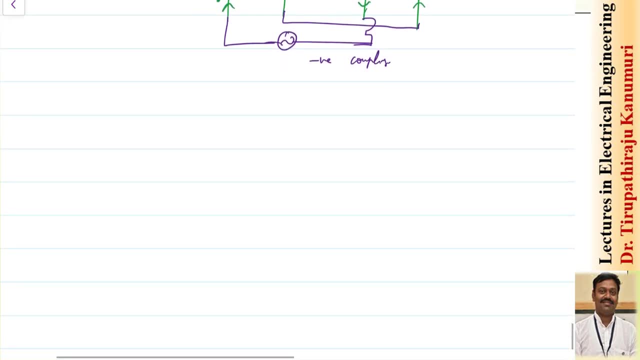 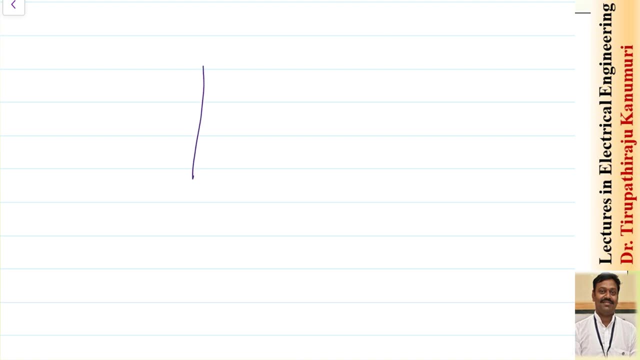 This can be returned to the supply. I hope to here it is clear to you. So now let us conclude and go for the basic construction of a transformer. So the transformer: In order to construct a transformer, there should be an iron core, Because the iron core or the iron material have high permeability, or the relative permeability. 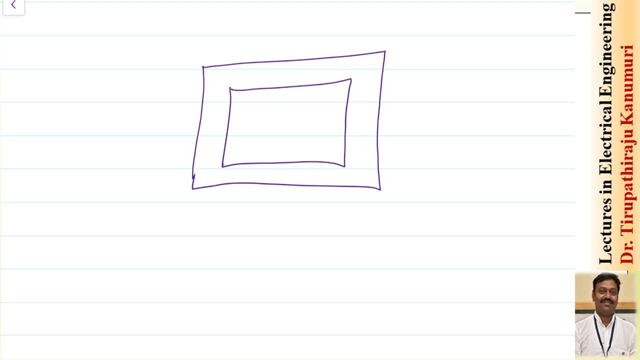 of the iron core is more. That means more magnetic flux can be produced for a given magnetizing component of current. That is the advantage of the iron core and particularly out of the iron core generally we go for the silicon steel and the silicon steel will be generally laminated silicon. 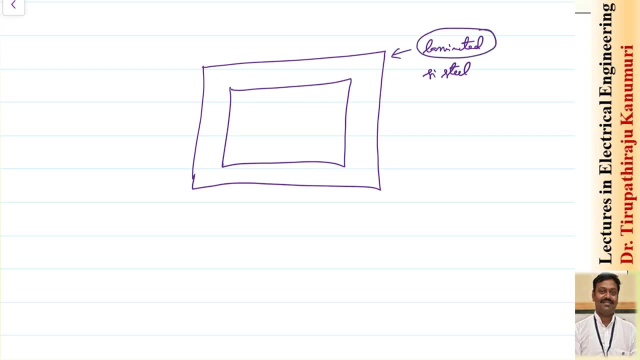 steel is used. So this lamination is used For decreasing the eddy current losses. we are going to discuss about these losses in the coming sections. So we go for laminated silicon steel. The advantage of the silicon steel is the permeability is. more it produces, the more 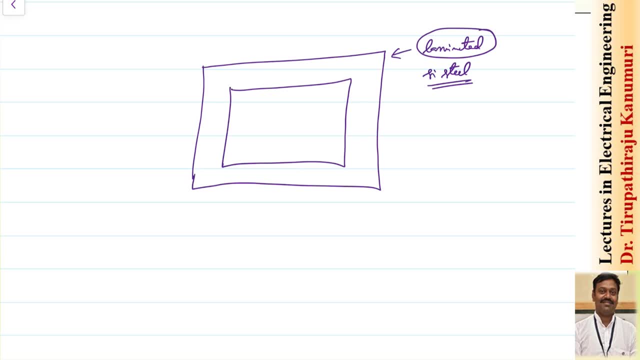 flux for a given magnetizing component of a current. It takes minimum magnetizing component of current. and the second advantage is the BH curve that comes. the BH curve will be very narrow in the case of the silicon steel, So automatically the hysteresis losses also will be minimum in the silicon steel. 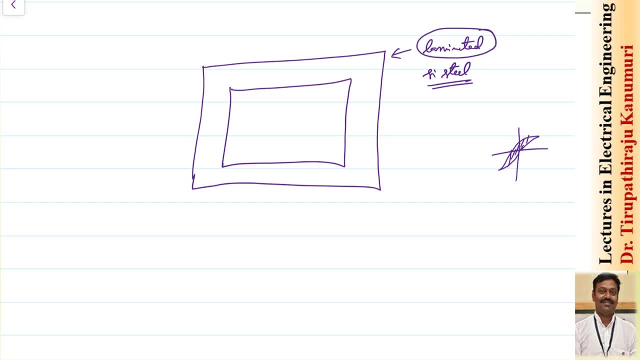 So this is the advantage of the silicon steel. This is the advantage. So now, along with this cue, there should be two coils connect the two coils. So this is one coil and this is my second coil. so this two coils are only magnetically. 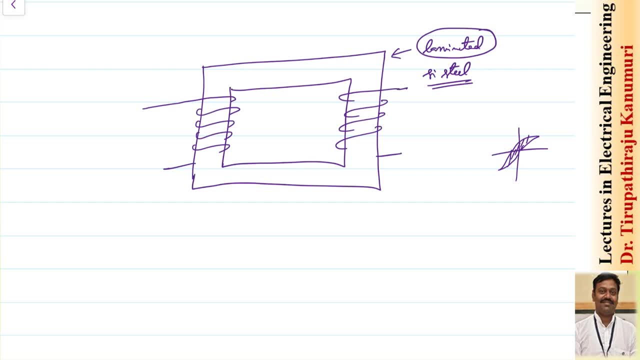 Tom made 爆, but they are not connected electrically together all this way. the coil which is connected to supply, So this is called as the primary coil, and the coil that is connected to the load, That is called mask secondary coil смог. 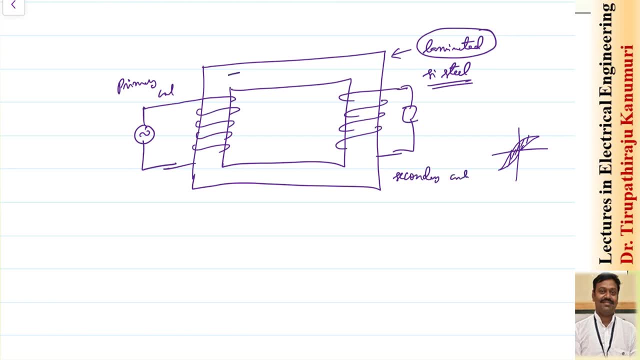 0.5 порядy delt away It. that means the basic skeleton or basic construction of a transformer will be: it will have an iron core or a common magnetic circuit and on this common magnetic circuit two- minimum two- coils will be wound. one coil will be the primary coil, which is responsible for the excitation or connected to 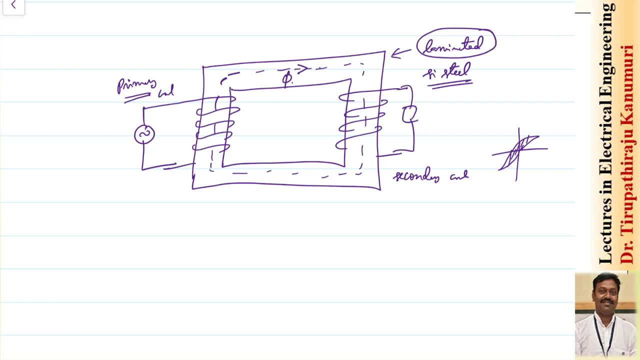 supply. one produces the flux phi in the core time varying flux. so this flux will link both the primary as well as the secondary. so emf- self-induced emf- will be induced in the primary coil and the mutually induced emf will be induced in the secondary coil and the energy is transferred from.